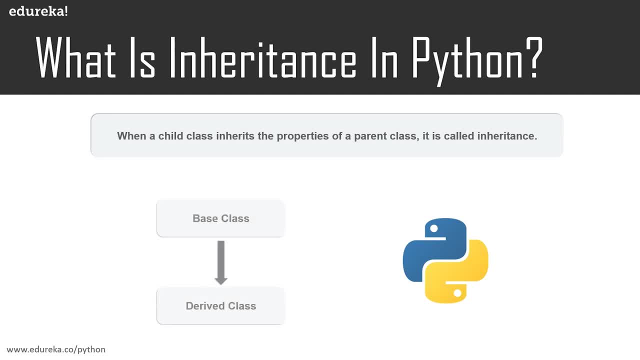 So, looking at it from the programming point of view, inheritance is when a class inherits properties from another class. the class which inherits the properties is known as a child class or the derived class, and the other class is known as the parent class or base class. Now let's take a look at a few advantages. 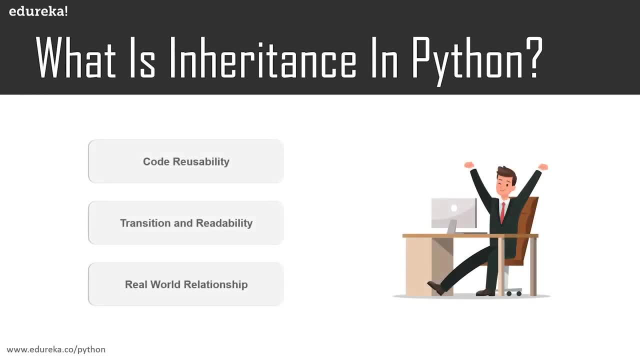 of using inheritance in python. So first of all, it is mainly used for code reusability, so that you don't have to write the same code again and again, and it provides a transitive property and also resembles a real-life relationship between classes. 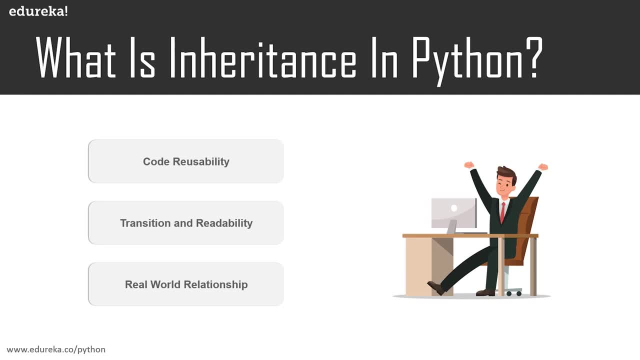 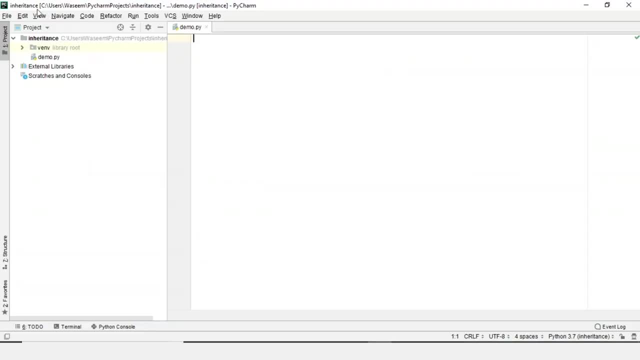 So these are the advantages of using inheritance in python, guys. So let me take a simple example to explain what is inheritance and how you can do it in python. So let's take it up to pie charm, guys. And now I'm going to enter the presentation mode. 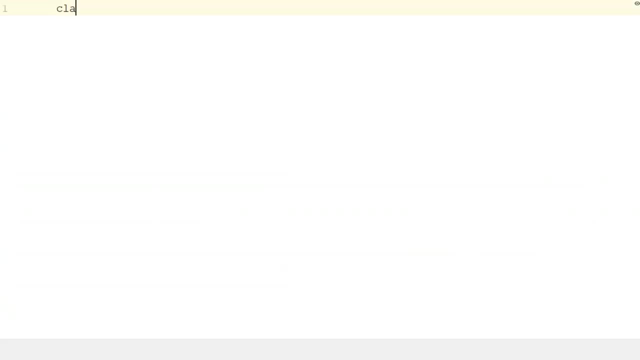 for better visibility. So now what I'm going to do is I'll just take one class guys and name it as parent. Let's say, now give it a function, So I'll name the function as function one, And after that let me give it a statement. 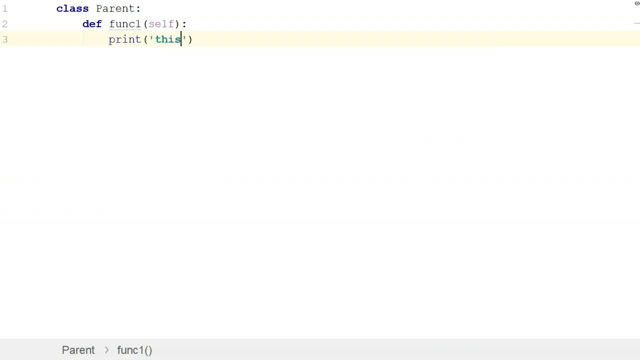 Let's say print function number one. Okay, let's say this is a parent function. Now what I'll do is I'll take one more class guys And name it as child, and for this, in the declaration I have to specify this parent over here. 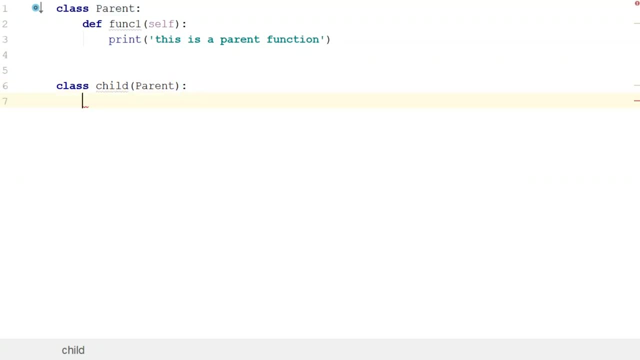 This is also known as subclassing. guys, We do the subclassing because a child class is not able to identify which class it is inheriting the properties from, so we do this by declaring the parent class inside the declaration of the child class. only now what I'm going to do is 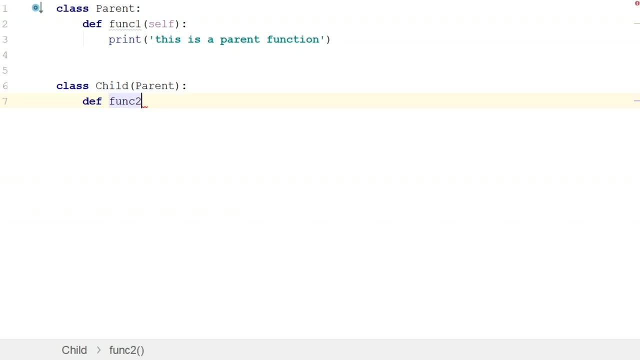 I'll just make one definition of a function. Let's say function number two, And in this I'll give the print statement, as let's say: this is a child function. Now, when we are declaring a child class, it must understand from which class it is inheriting. 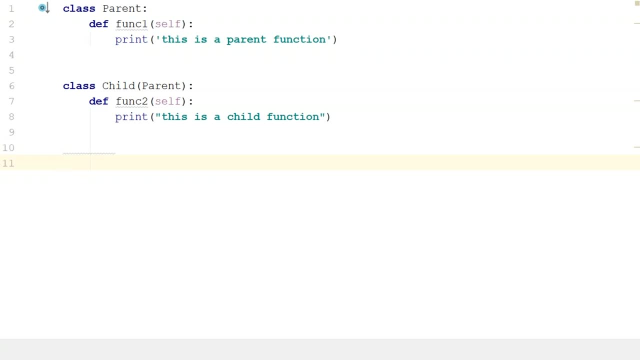 the properties from. so we have declared the child class with the parent class in the declaration, and that's how the child class differentiate between a parent class guys. So now to call the parent class methods, use the child class objects. What I'm going to do is I'll just make an object. 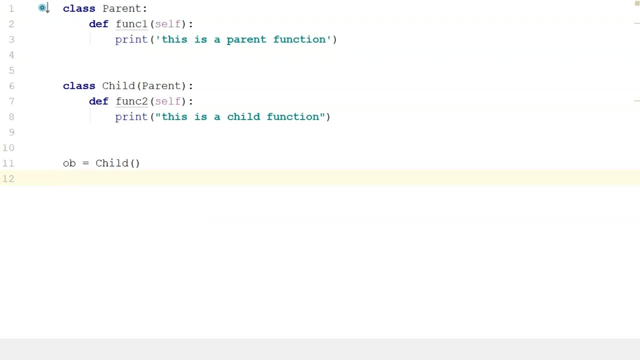 of the child class guys now to call this parent function, which is the function number one. Let's see if I can do that. and I'm getting function 1 and function 2 as well, So I can call both the functions. So first of all, I call the function 1. 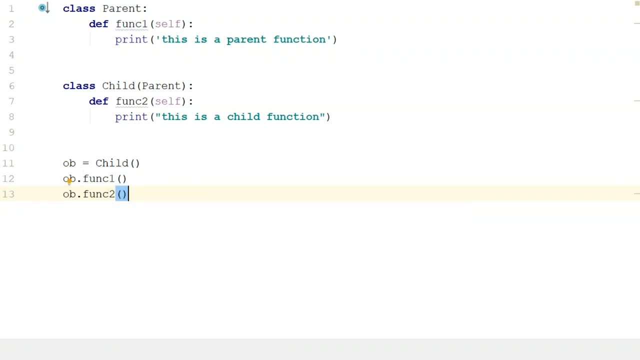 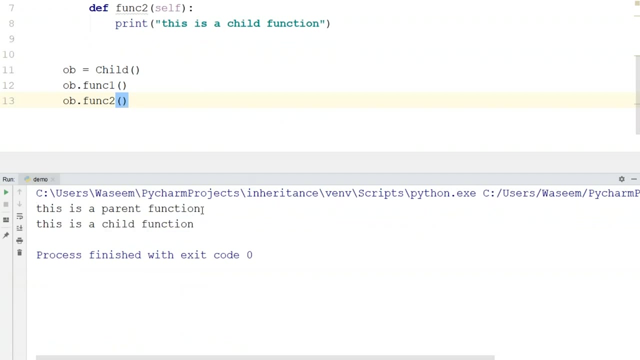 and after that I'll call the function number 2.. Let's see what the output will be. Now the output is: this is a parent function and this is a child function. So, basically, what we have done is we have taken two classes, named it as parent and child. 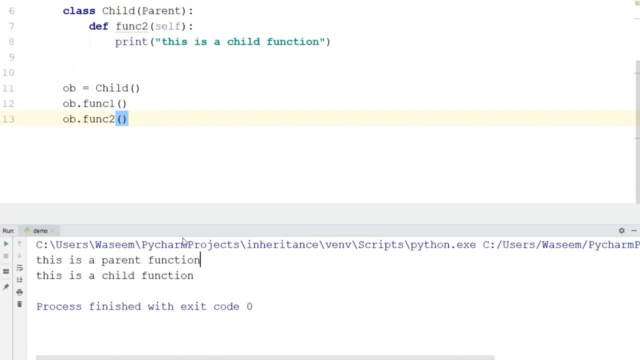 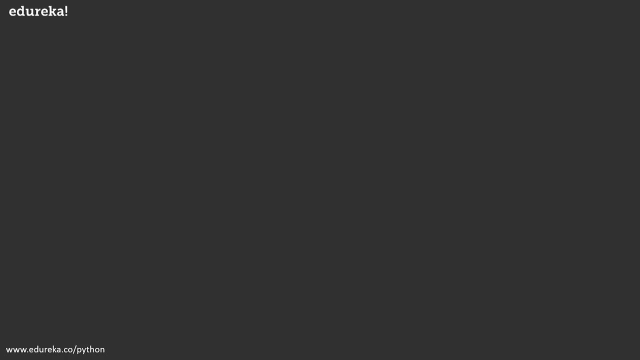 and from the child class, we are inheriting the properties- These of the parent class here, which is the function number one, and this is the basic example of inheritance. guys, This is how you can do it, Now that I've shown you a simple example. 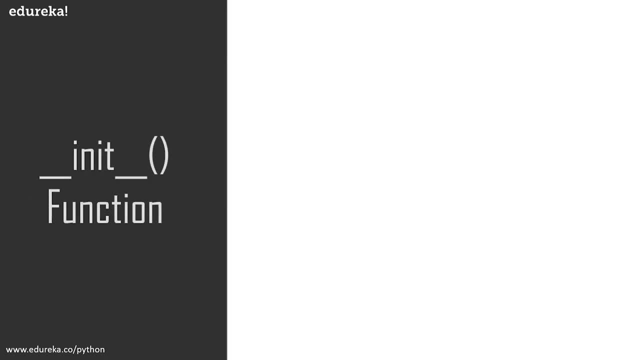 Let's talk about the innate function in Python. So what exactly is a unit function? in it, function automatically gets called each time an object is created for a class. now, when we add a unit function to a parent class, a child class will not be able to access the parent class method. 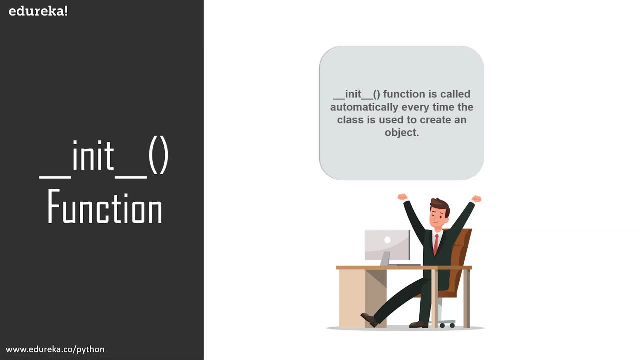 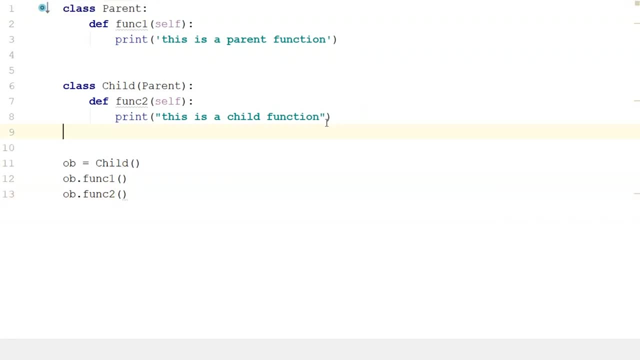 So to overcome this, the child class in it function overrides the parent class in it function. So now let's take a look at an example to understand this. now to show how in it function works, Let me first clear this. We'll write a in it function over here. 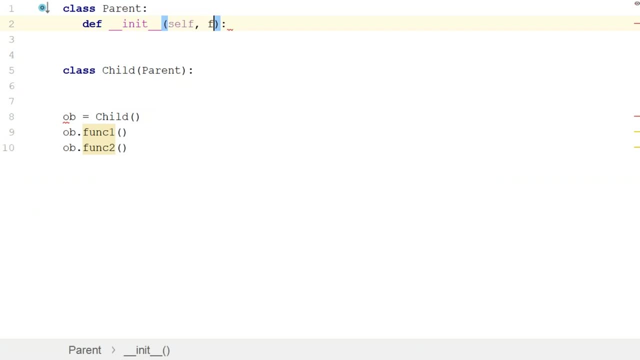 Yes, and instead of self I will add one more variable, Let's say F name and F H. now what I'll do is I'll just write: self dot name is equal to F name and self dot age is equal to F H. Now I'll take one more function, guys. 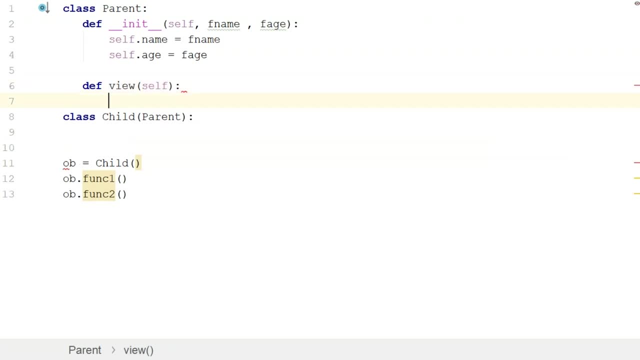 So I'll just name it as, let's say, view, and for view I want to print the value of F name, Self dot name and self dot age. So this is my parent function guys. and for the definition in the child class I will also make one in function. 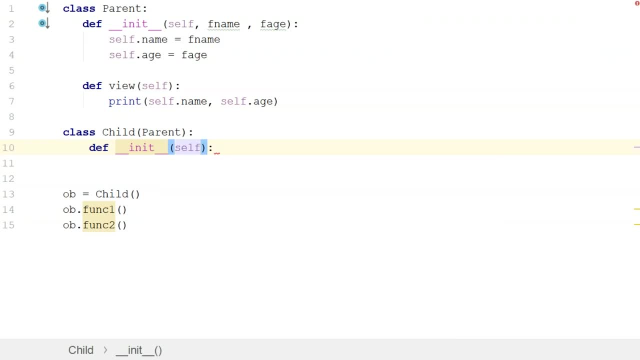 So I'll just write it as in itself, And again I have to add F name and F age And let's say a self dot name is equal to F name and self dot age is equal to F age. Now this in it function is going to overwrite the parent. 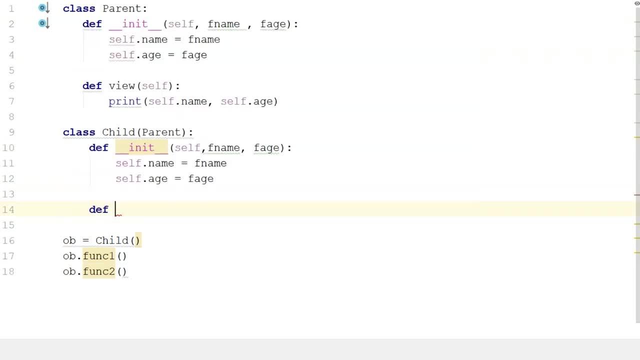 in function guys. So let's make one more function. So this is going to be view as well, And in this let's say I want to print: okay, before we move on, We have to specify the parent function with the unit function as well. 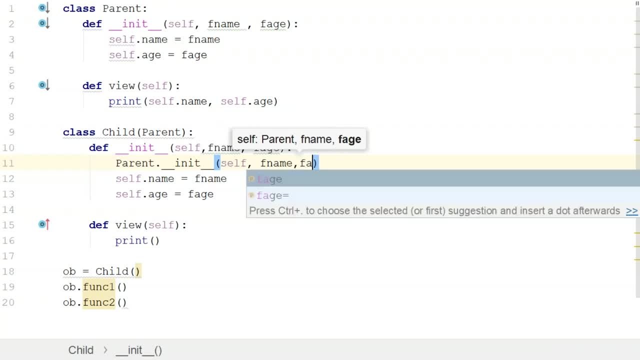 So I'm going to add one more, And we don't have to mention these variables. instead, I'm going to add one more. Let's say, I want to add last name as well, And I'm going to add it as, let's say, Eddie Raker. now, 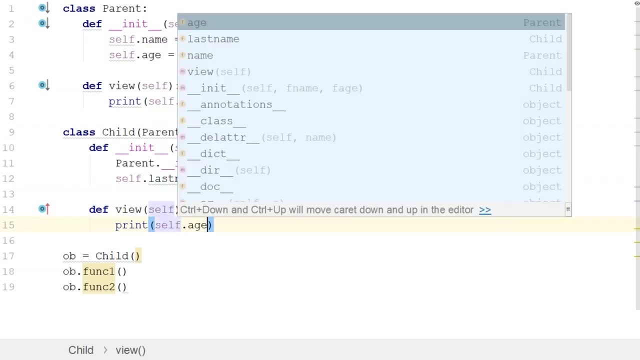 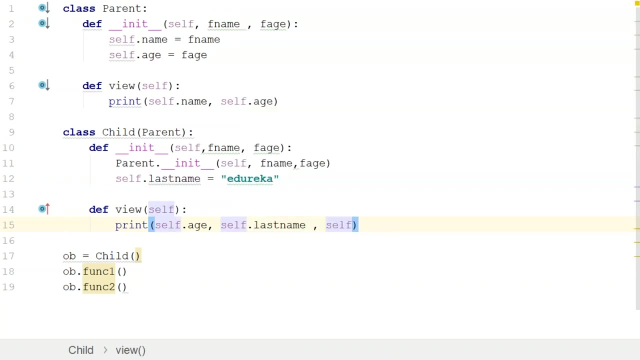 I'm going to print over here: self dot- age, Self dot- last name and self dot. Let's say name. All right, I have to remove these. let's make one more object And give it the value. Let's say: I want the age to be 23. 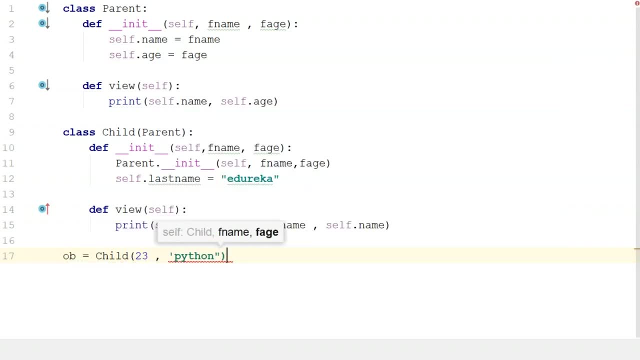 and last name is going to be python In the inverted commas name We have already specified, so we don't have to give it again, and I'm going to just call the function. Let's see what happens. What is output will be so, as you can see, I'm getting the output. 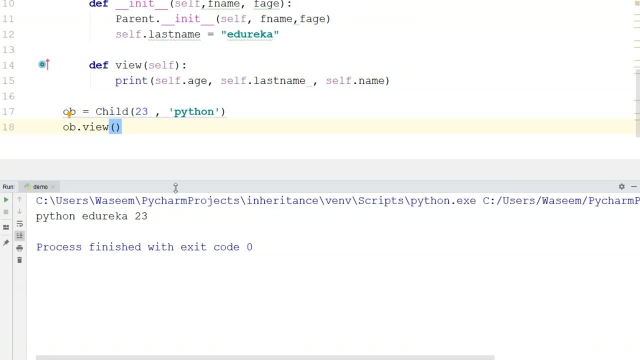 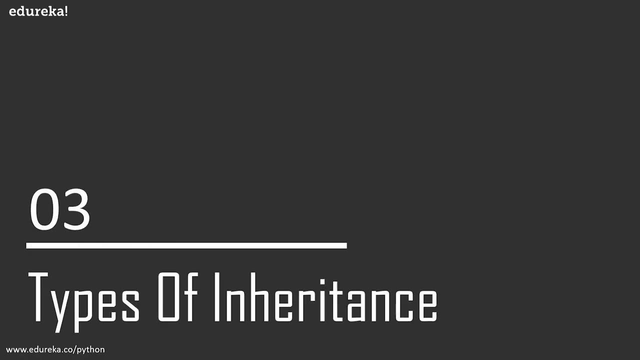 As python and Eureka and when you see. so this is how you can override the parent class in it method using the child class, guys. So this is all about the unit function. Now let's talk about the next topic that we have, which is the types of inheritance. 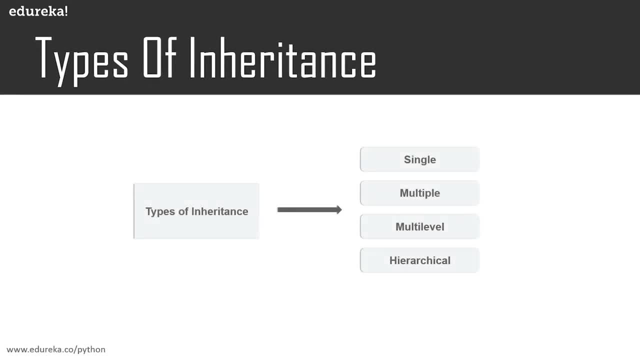 So depending upon how many types of parent class and child class are going to be there inside the program following other types of inheritance in Python guys. So there is single inheritance, There is multiple inheritance, Then there is multi-level inheritance, hierarchical inheritance and there is hybrid inheritance as well. 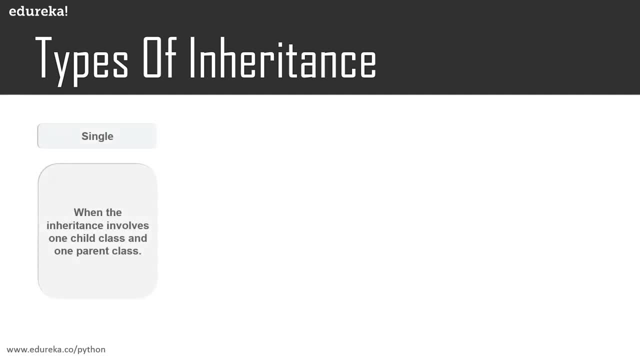 So we're going to talk about each of them in detail, guys. So first of all, let's talk about what is single inheritance. So when the inheritance involves one child class and one parent class only, it's going to be a single inheritance. The example that I showed you before is the example 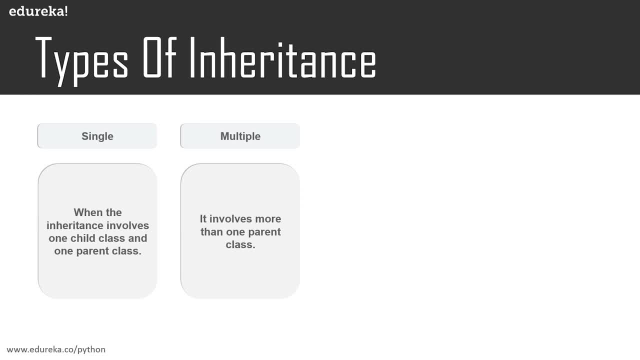 of single inheritance guys and talking about multiple inheritance, It is going to involve more than one parent class, which means we are going to have at least two parent classes and the child class is going to derive properties from both of them, And this is called multiple inheritance. 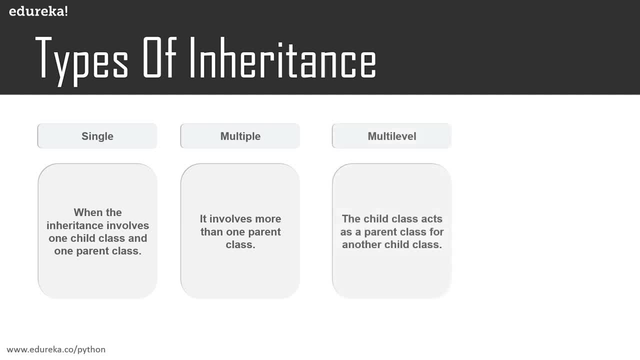 Now talking about multi-level inheritance, Let's say we have a single inheritance going on. We have a parent class and we have a child class, but the child class also act as a parent class for another child class. that is going to be a multi-level inheritance, guys. 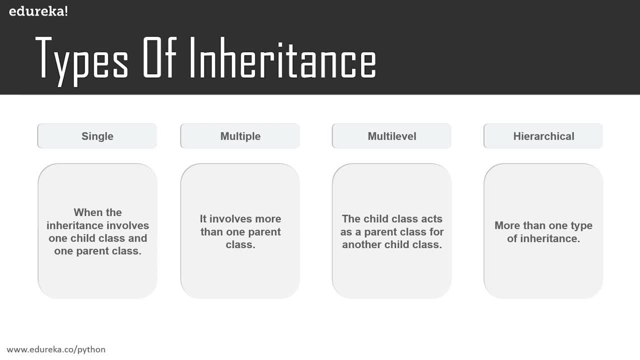 and talking about hierarchical inheritance. hierarchical inheritance actually involves multiple inheritance from the same parent class. and talking about hybrid inheritance: If a program has more than one types of inheritance, let's say we have a single and multiple inheritance going on simultaneously. It's going to be a hybrid inheritance, guys. 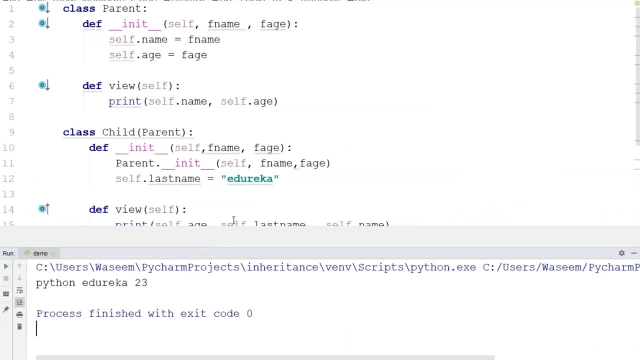 So let's take a look at examples for each of them. So let's go to pie charm, guys, and I'll remove all this. So let's start with single inheritance, guys. So I'll just take a parent class And give it a function. 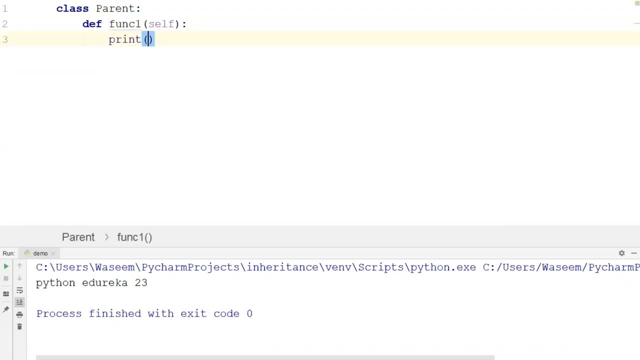 Let's say function one And give it a statement. Let's say: this is function one. Now let's take another class- guys, class child- and give it the value of the parent class, and after that we can move for another function. Let's say function number two and give it a statement. 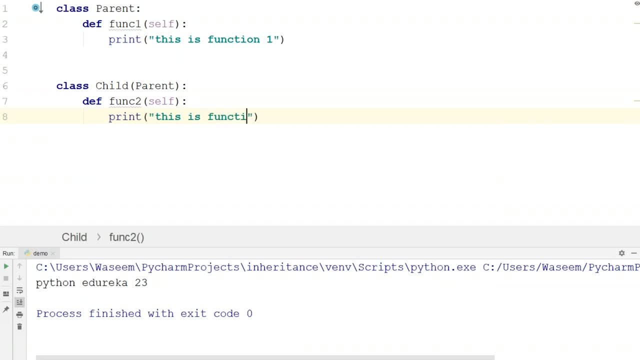 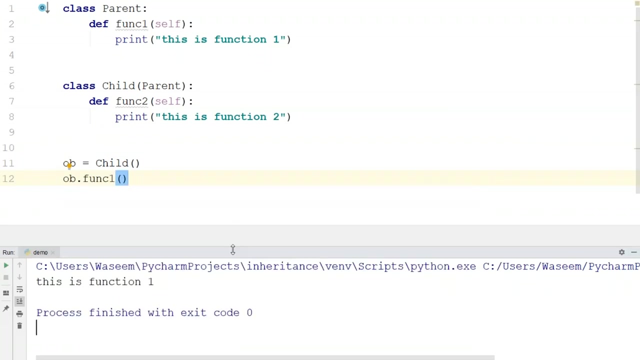 Let's say print, This is function. to now make a child class object And call the function, so we can call both of these functions. So just call function one, give it the output and we are getting the output, as this is function one. So this is a basic example of single inheritance, guys. 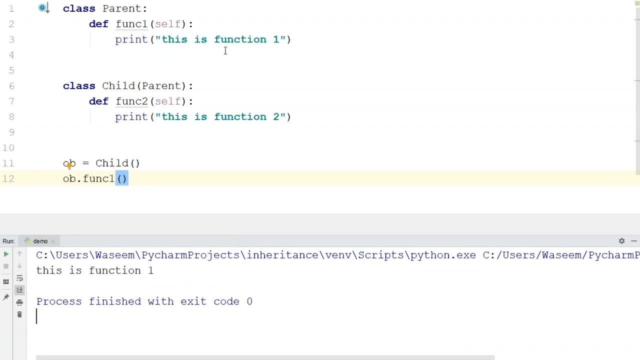 not talking about multiple inheritance. What I'm going to do is I'm going to make one more class over here. Let's say: class parent to. now what happens here? Let's say: give it a function number three. Let's say: and print statement. 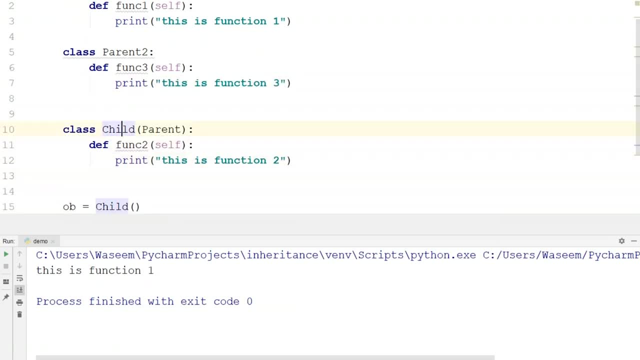 This is function three, and in the declaration over here I'm going to just specify two classes, and when I call the functions, I can call function number one and I can call function number three as well, guys. So let's see what is happening here in the output. 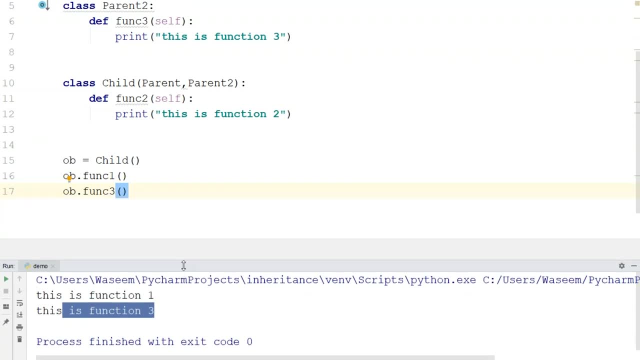 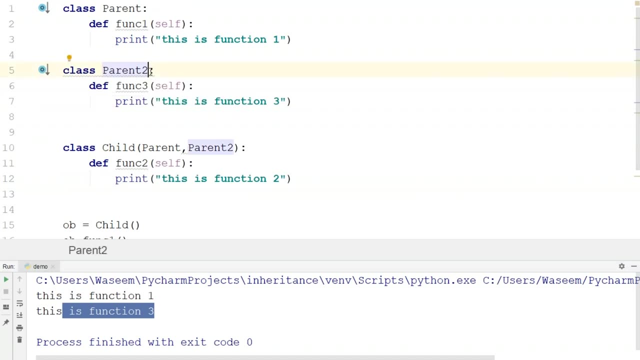 I'm able to call the function number one and function number three as well from the child class object. So this is the example of multiple inheritance, guys not talking about multi-level inheritance. So what I'm going to do is I'm just going to specify parent. 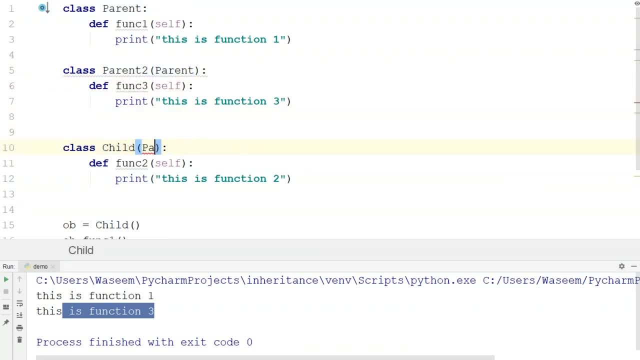 over here and from this, let's say, it doesn't have any declaration of parent one which is this class, So it is not able to inherit any properties from that. But what I'm going to do is I'll just specify parent two over here. 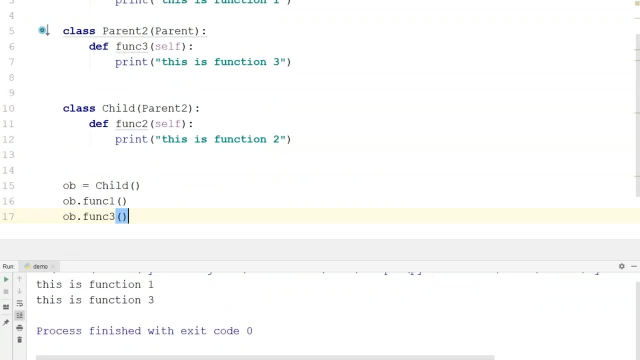 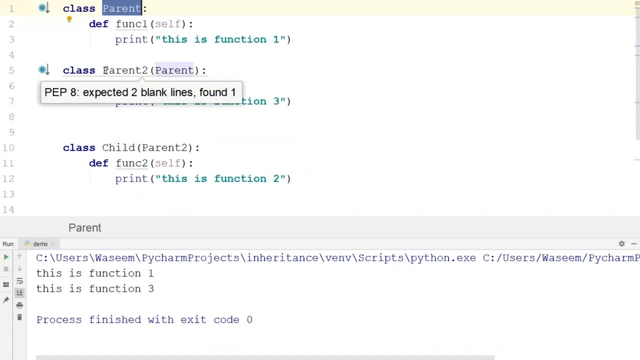 And I can still call these functions because there is an inheritance going on between them, which is multi-level inheritance, which basically means this class, the parent one class, is actually giving properties to parent to class and parent to class is giving properties to the child class. 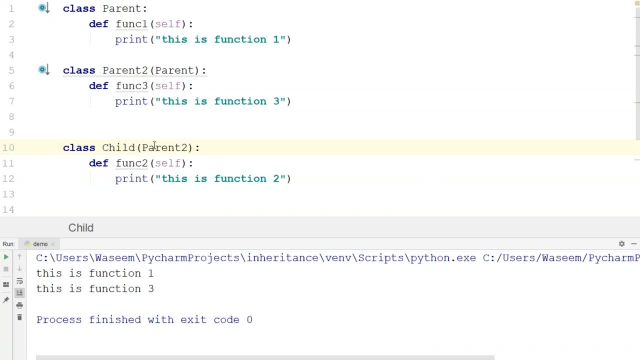 So this is example of multi-level inheritance guys, not talking about hierarchical inheritance guys. What I'm going to do is, instead of parent two over here, I'll just specify parent. So for these two child classes I have the same parent class. and now let's see. 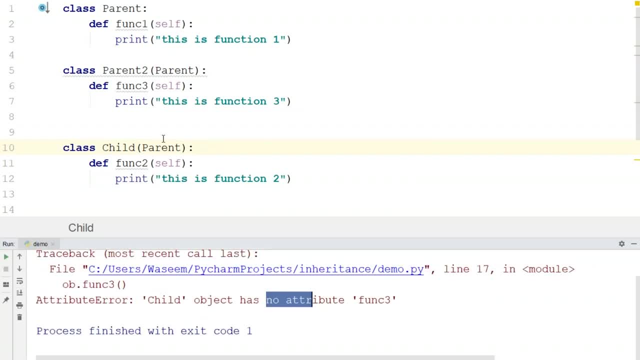 if I can have the same output or not. I'm not going to get the properties from the parent to because I have not specified it in the inheritance, So I'll just remove this and let's see what happens. I'm getting the output. 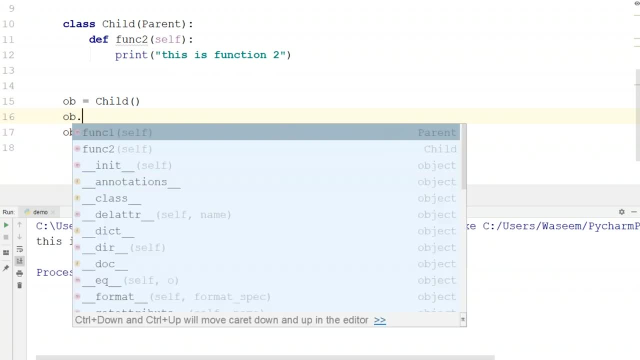 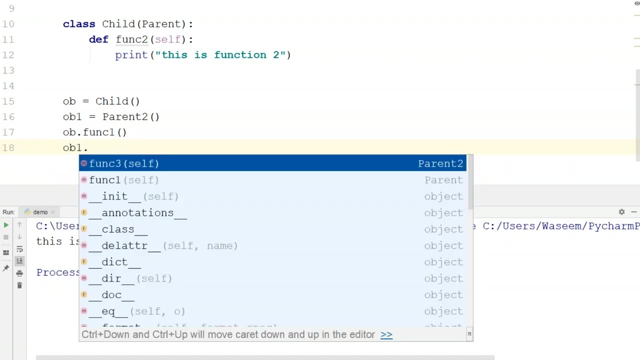 This is function one. Okay, let's make the object for parent two as well. All right, give it one and OB one dot. Let's say what functions we can have. I can have the function number three and I can have the function number one as well. 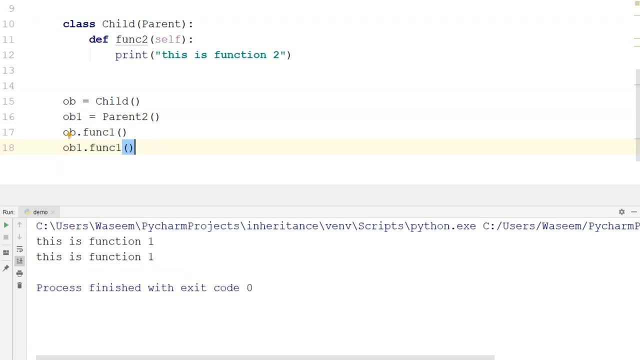 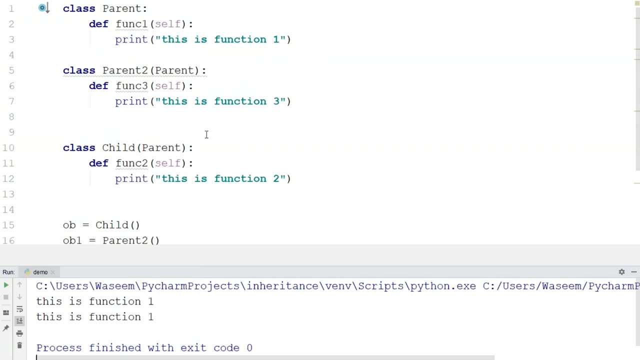 So I just print function number one and from both the child classes I'm able to print the function number one. So this is the example of hierarchical inheritance. guys, I'm using the same parent class to give the properties to both parent to and child class as well. 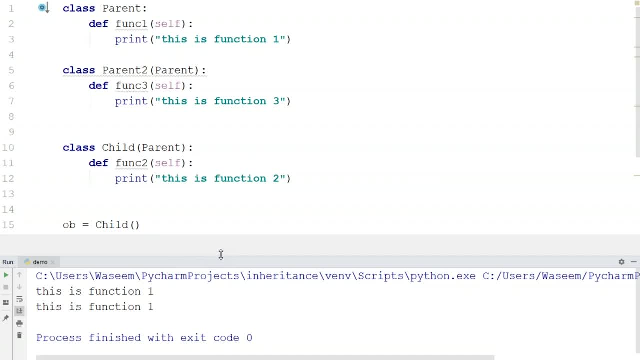 And now talking about hybrid inheritance. hybrid inheritance actually involves more than one inheritance going on in the single program. So we have a single inheritance over here. So let's say, I want to have multiple inheritance as well. So I just specify parent to now. and this is the example of hybrid inheritance, guys. 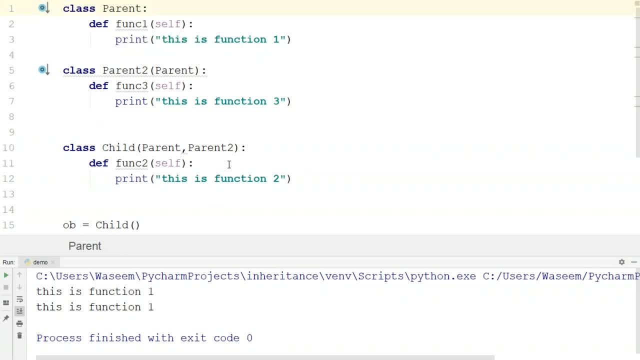 Because we have a single inheritance going on over here and in the child class I'm inheriting both the parent one and parent two, and this is the example of multiple inheritance. So this is a hybrid inheritance example, guys, Okay, we are getting a type error. 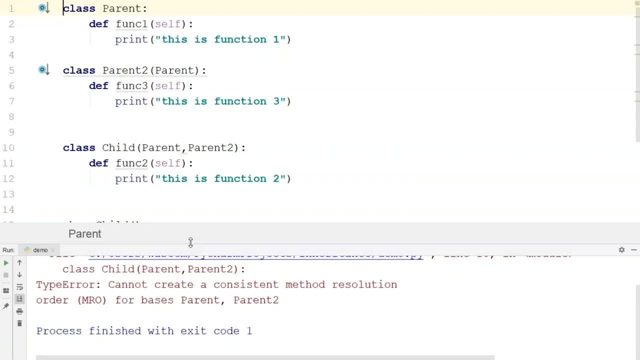 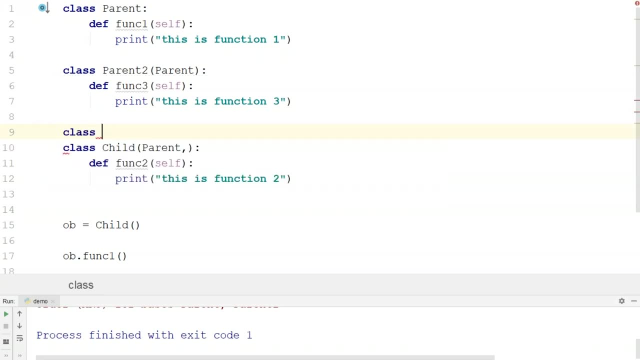 which is saying: cannot create a consistent method resolution order for base parents, parent one and parent two. Let's say instead of this: I'll make one more class over here. Give it a value. Let's say, parent number three, Give it a function, function. 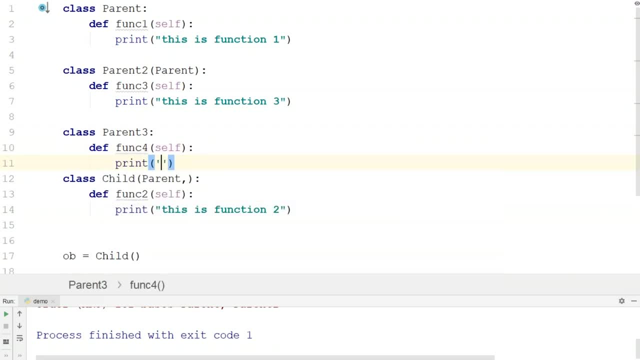 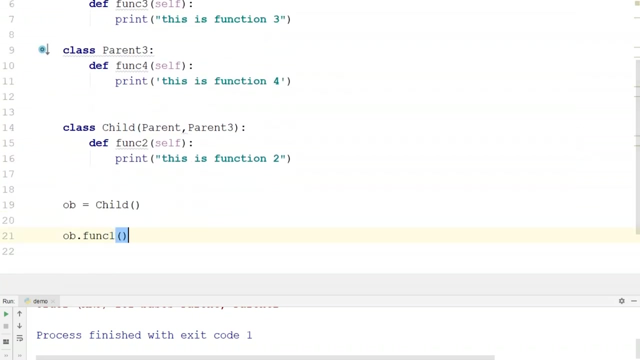 Let's say four and print statement. This is function for now. instead of parent number two, what I'm going to do, I'll just take parent number three guys, and with the child class operator, Let's see if I can actually get the function number one. 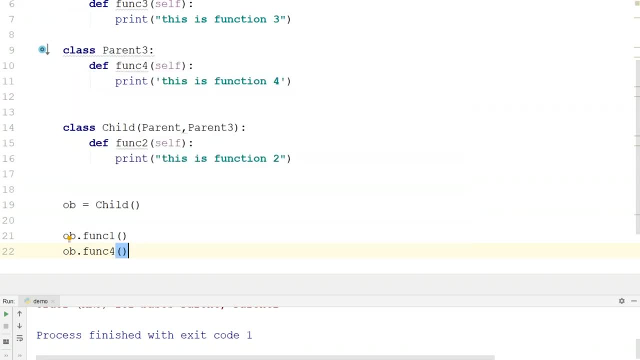 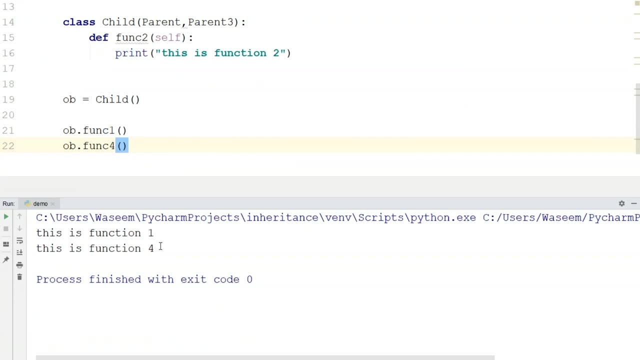 and let's say, I want function for as well. I'm able to do that. So in the output let's say what I get. I'm getting the function one and function four. So this is a simple example of hybrid inheritance. guys, now 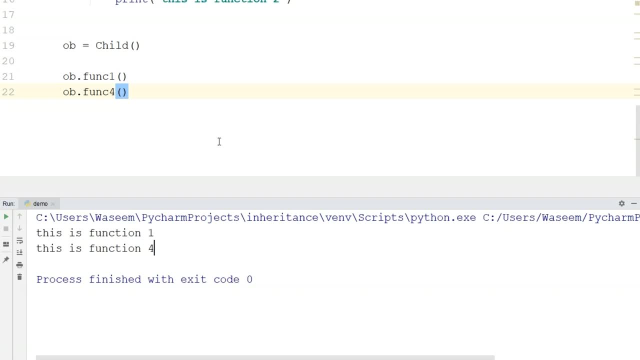 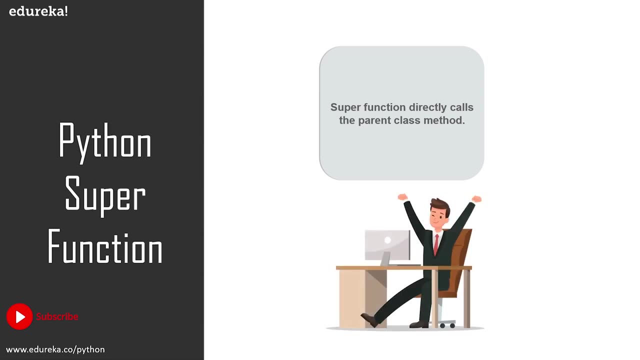 that we are done with the type of inheritances. Let's take a look at what all we have now. So we're going to talk about the super function, guys. super function actually calls the parent class method directly. So let's take a look at a simple example, guys, how it works. 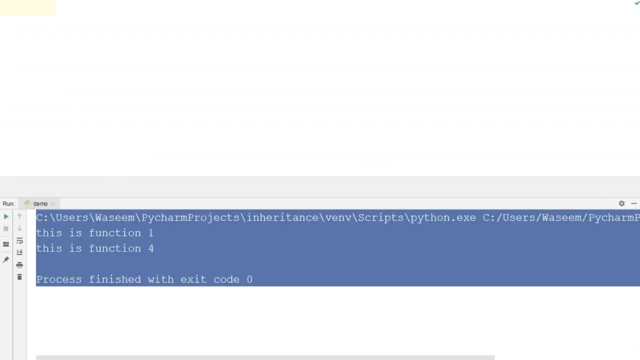 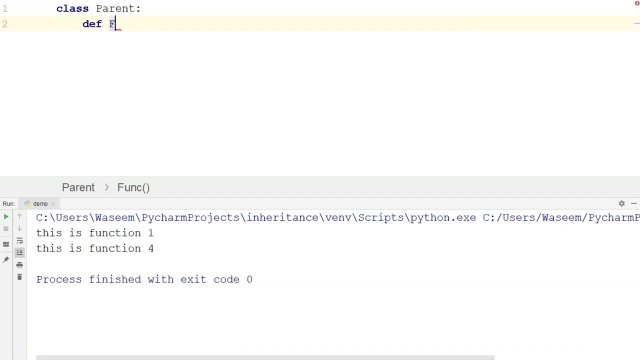 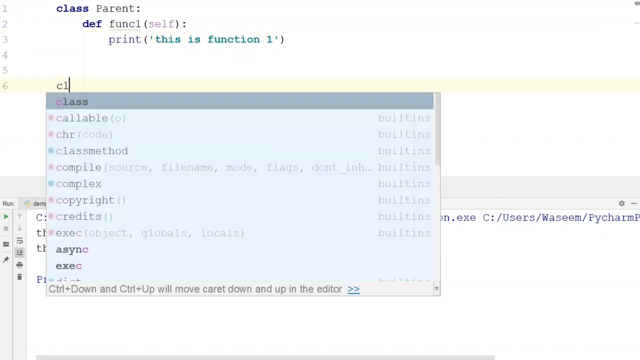 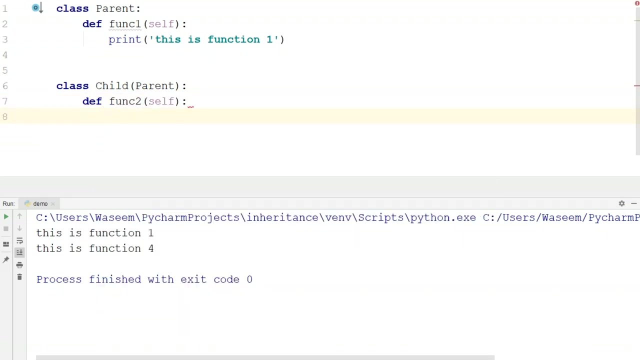 So I just remove all this. Now what I'll do is I'll make a, let's say, parent class And give it a function function, one Again, the print statement. Now what I can do is, instead of calling the parent function from the object, 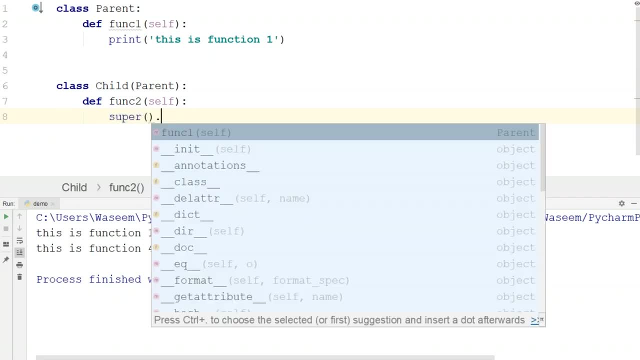 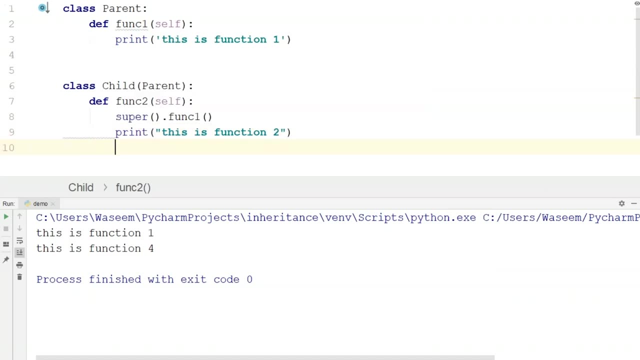 I can just use the super function and over here I can just call the function one. now I'll just print: this is function to. let's make a child class object. Now let me see if I can call the function to or function one. 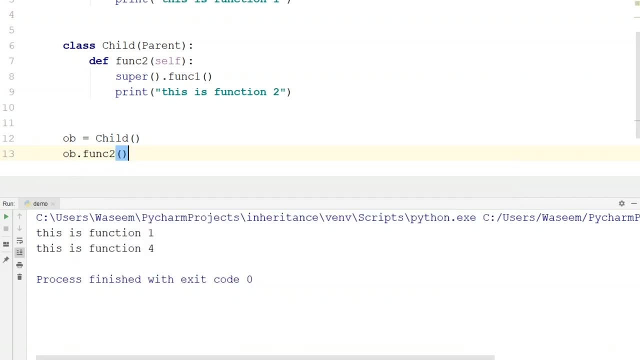 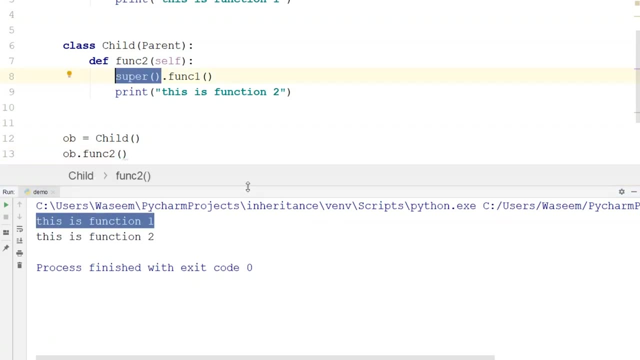 I can do that. So I'm going to call the function to race. Let's see what the output will be. So I'm actually able to call the function one directly from the super function over here. So this is the function of super function guys. 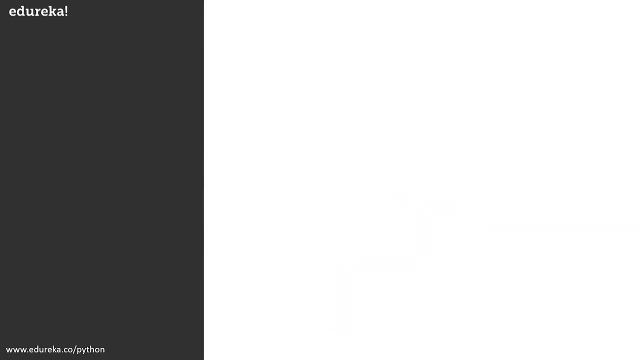 It can directly call the parent method. and now that we are done with the super function, Let's take a look at the next topic that we have, which is method overriding in python. So method writing can also be achieved if you change the functionality of the parent class function. 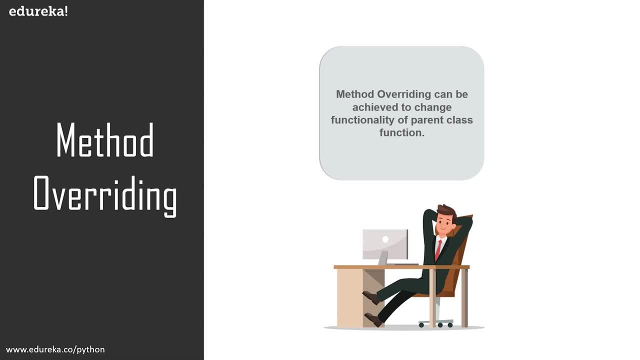 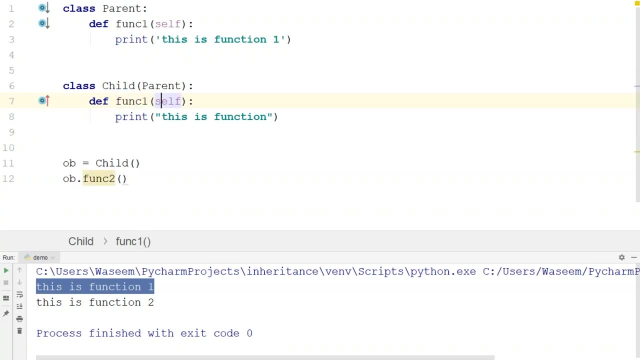 So let's take a look at an example to understand how we can actually achieve method overriding in python guys. So instead of naming them separately, I'll just name them as same. So when I create the child class constructor and if I call the function now okay, function one.